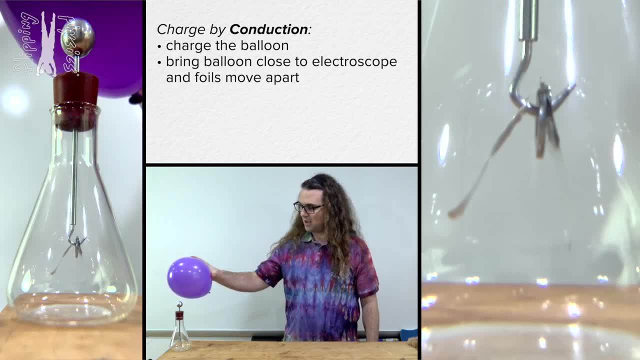 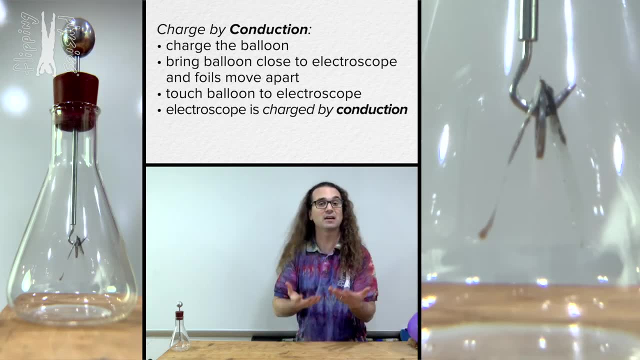 can see the foils of the electroscope begin moving apart, And then Then when I touch the electroscope, I have now charged the electroscope via conduction. So this is a charged electroscope via conduction and I can touch the electroscope with my finger. 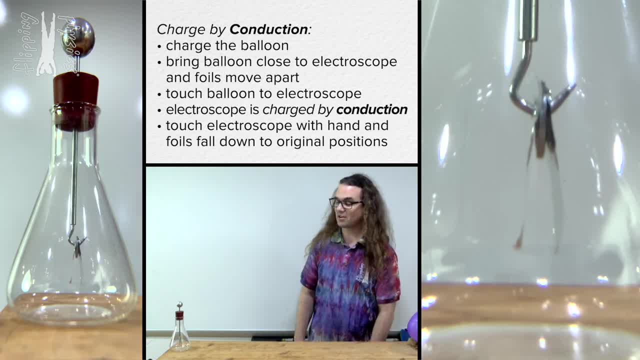 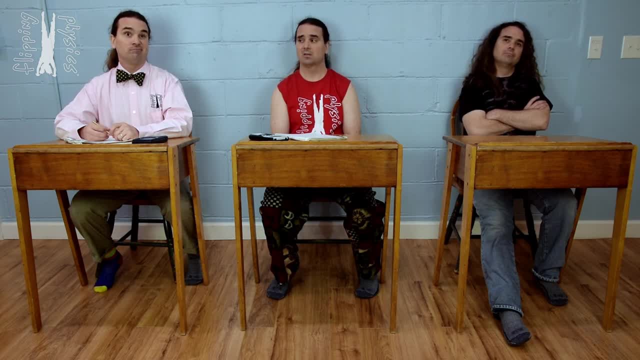 and the two foils move back to where they started. That's it. I'm glad to know we're going to walk through that step-by-step, because I have no idea what just happened. Right, That is not a problem, because we're going to go through it step-by-step. 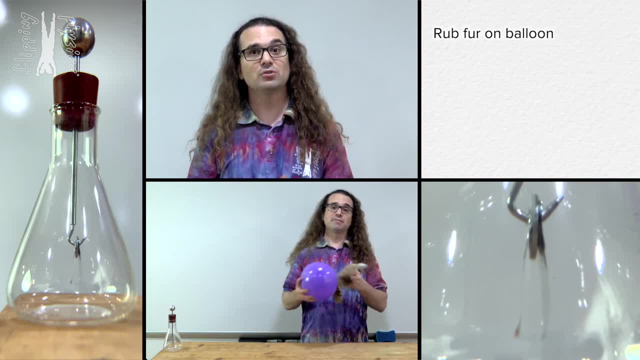 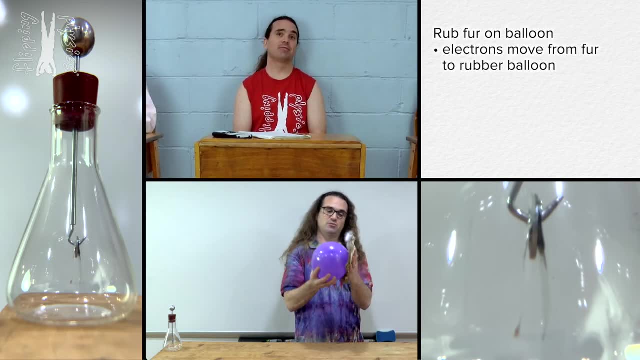 So let's start with the first step. Rubbing the fur on the balloon causes what to happen to the fur and the balloon. Bobby, Oh, I know that one from before. Electrons move from the fur to the rubber balloon, causing the fur to have an excess positive charge and the rubber balloon to have an excess negative. 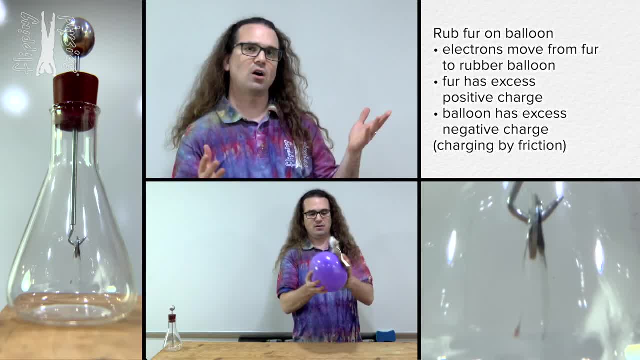 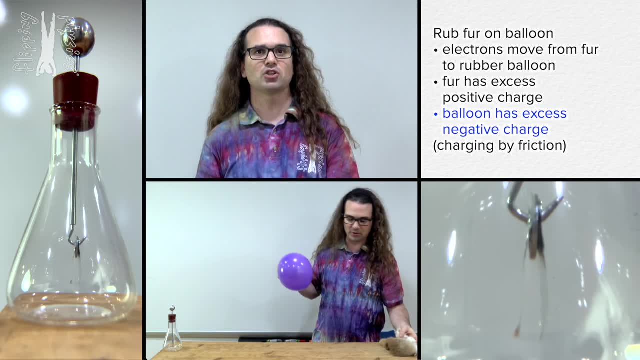 charge. I believe this is called charging by friction, Correct? Although at this point we really are only concerning ourselves with the net negative charge on the rubber balloon. The other object in the demonstration is the electroscope Bo. before I bring the balloon near the electroscope, what is the approximate net charge of the? 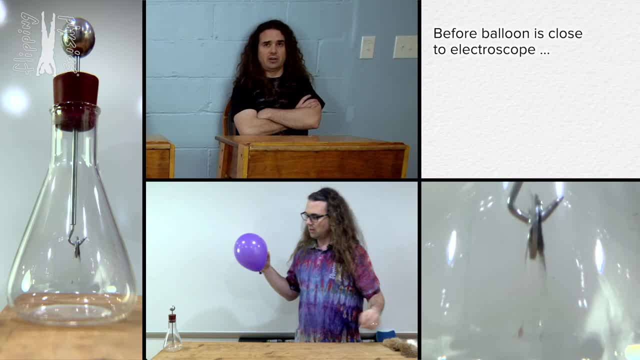 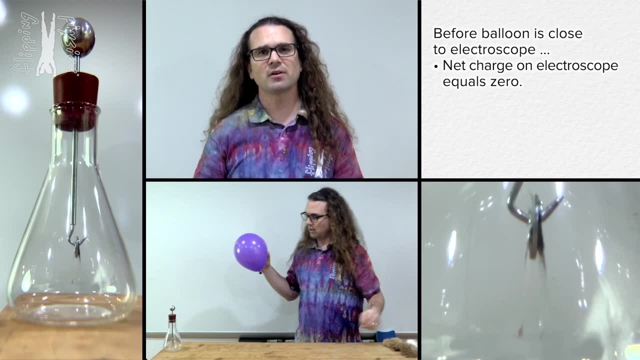 electroscope. Well, Before we start, the electroscope should have a net charge of zero. It should have a neutral charge, right, Right? So before we bring the two objects near one another, the electroscope has roughly an equal number of positively charged protons and negatively charged electrons, And the 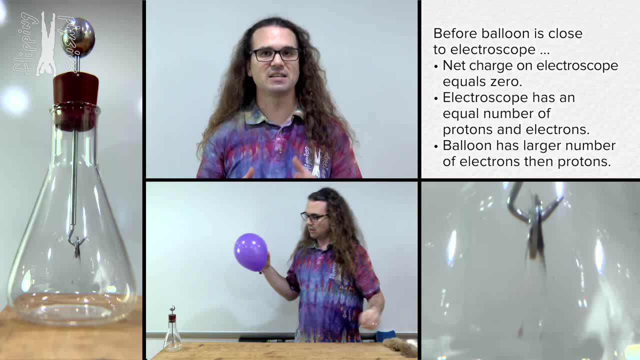 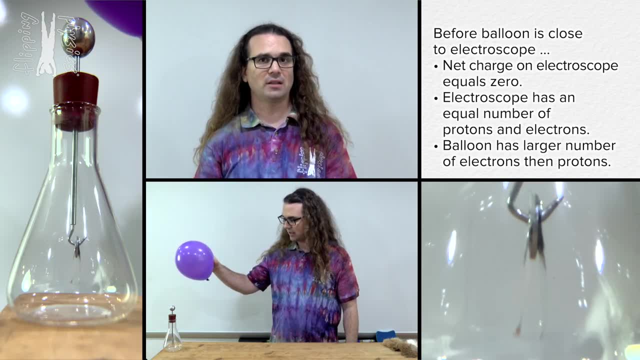 balloon has a larger number of electrons than protons, giving it a net negative charge. Now watch what happens as I bring the rubber balloon near the electroscope. Even before I touch the balloon to the electroscope, the two metal foils at the base of the electroscope. 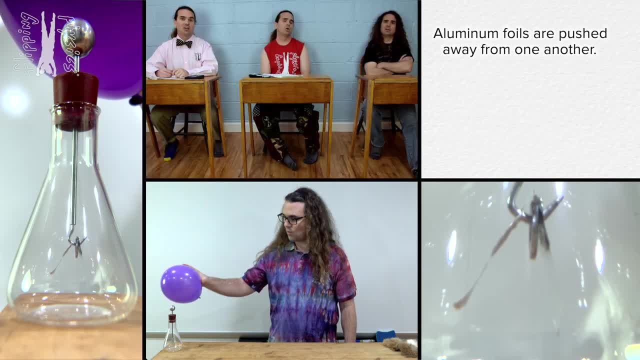 are pushed apart from one another, Bobby? why do you think that is? If the two metal foils are pushed apart from one another according to the law of charges, they must have the same charge and there must be an electric force pushing them apart. But 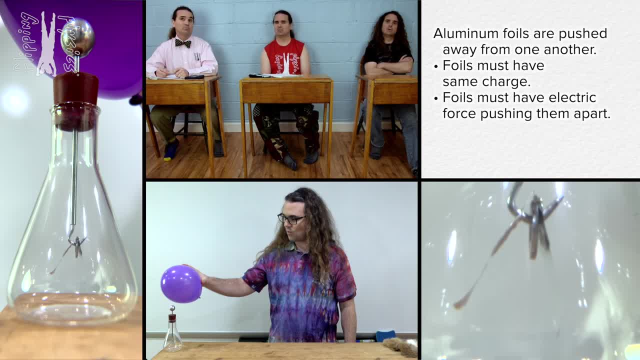 I do not know if the net charge on each of the foils is positive or negative. We can use the law of charges to figure that out as well. We know protons do not easily move because they are in the nucleus of the atoms. That means the electrons are the ones. 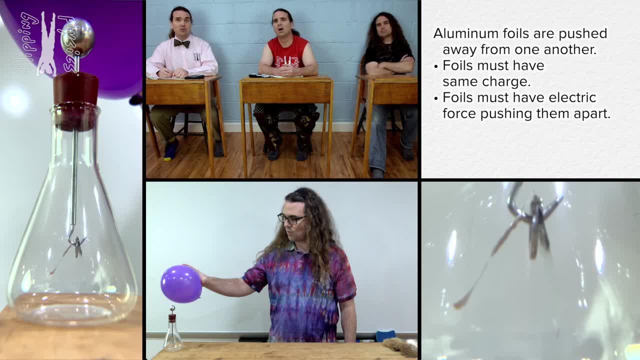 the ones that move. so the electrons in the electroscope which are negatively charged are repelled by the negative charges in the balloon and float down to the metal foils. That must mean when the balloon is brought near the electroscope the metal foils have 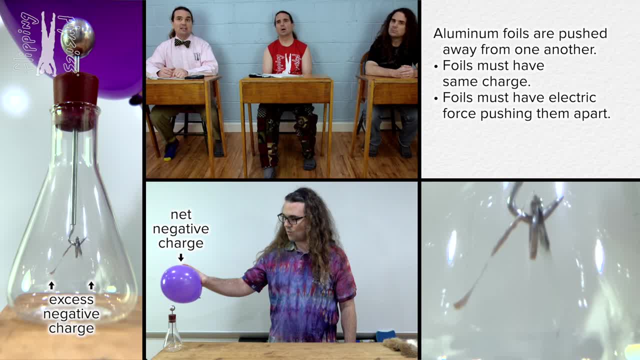 an excess of electrons or a net negative charge and an electric force pushes the metal foils away from one another. That means the top of the electroscope has a net positive charge because there are fewer electrons than protons in the ball at the top of the electroscope right. 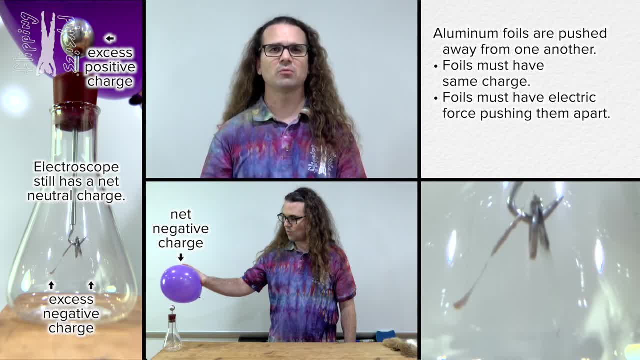 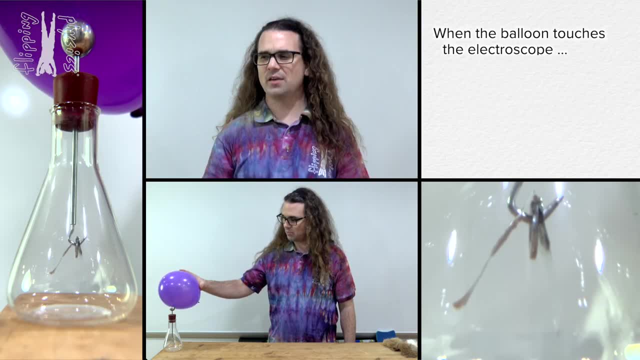 Mrp. Correct, Now we know what happens before the balloon touches the electroscope, But what happens when the balloon touches the electroscope? I have no idea, Mrp. I do not know. Mrp, Touching the two objects together allows electrons to transfer between the two objects. 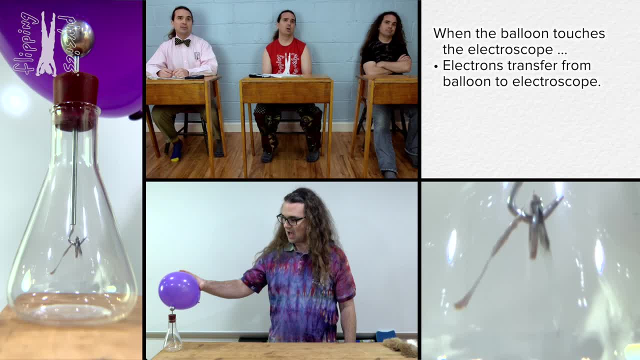 Oh, that means electrons will transfer into the electrically neutral electroscope from the balloon. That is because the electrons will be attracted to the protons near the top of the electroscope and repel the electrons. Mrp Right, They come from one another where they are crowded together, close together in the balloon. 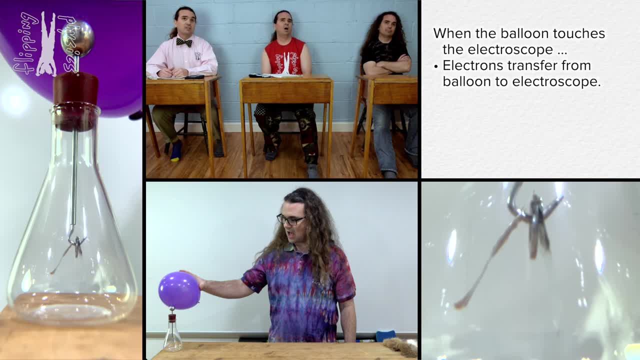 Because the rubber balloon transfers some electrons to the electroscope to balance out the net negative charge. both the rubber balloon and the electroscope end up having some excess electrons, But the total number of excess electrons in the balloon-electroscope system remains the same, because the total number of electrons will stay the same. 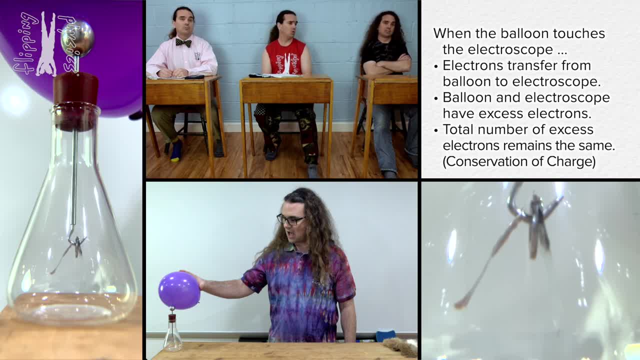 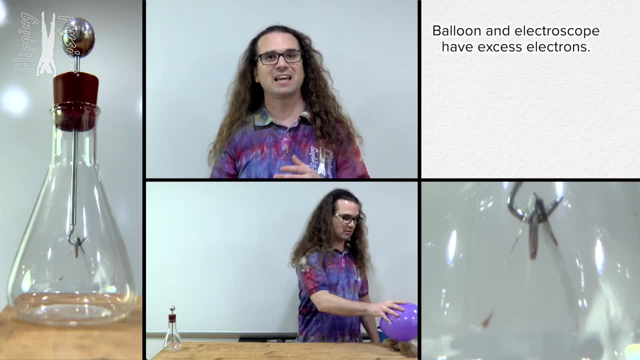 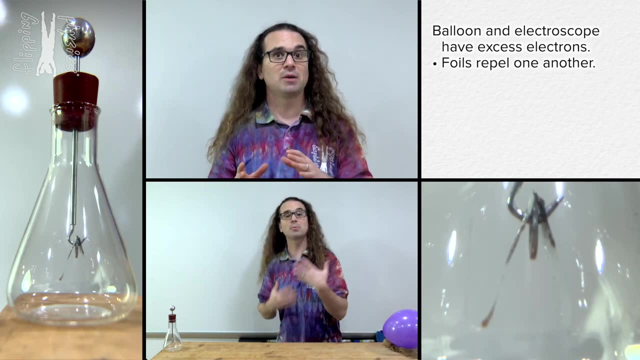 Conservation of charge. The total electric charge of an isolated system never changes, Mrp, Yep. At this point, then, both the balloon and the electroscope have an excess number of electrons, causing a net negative charge, Which is why the metal foils of the electroscope remain repelled from one another. again because 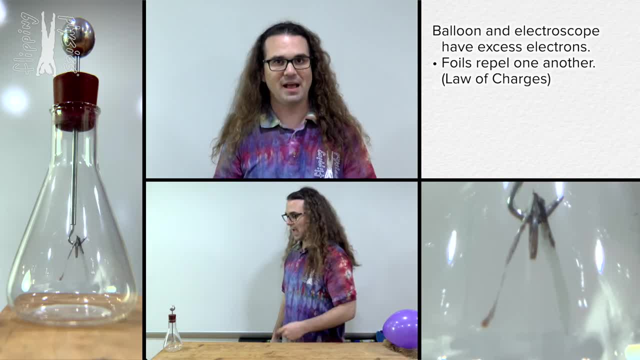 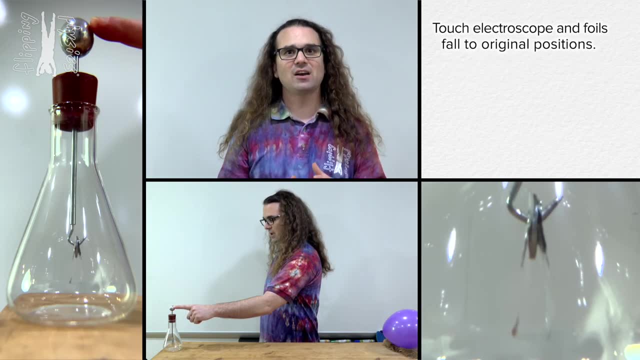 of the law of charges. Like charges repel Again. at this point the electroscope and the balloon both have an excess number of electrons. And then I touch the electroscope and that causes the foils to no longer be repelled from one another. 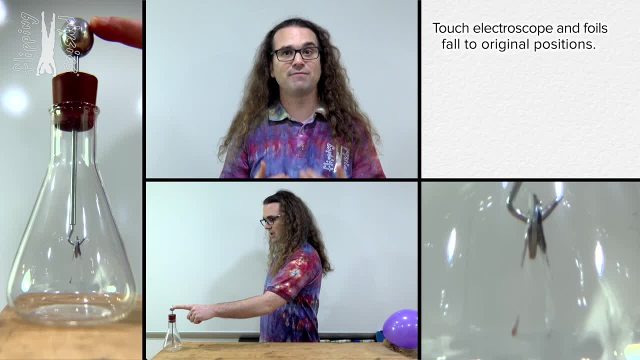 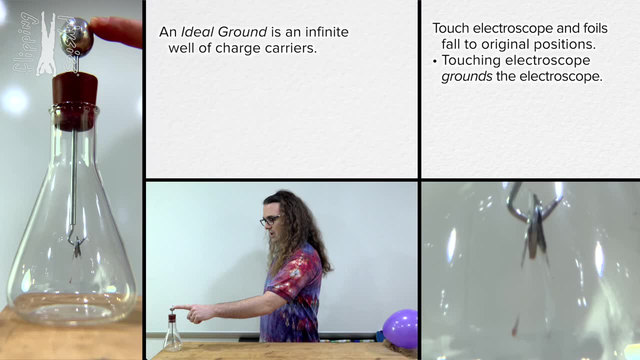 This is because, compared to the charge on the electroscope, the charge on the balloon and the electroscope, I have a very, very large number of charges and I act as a ground. An ideal ground is an infinite well of charge carriers. 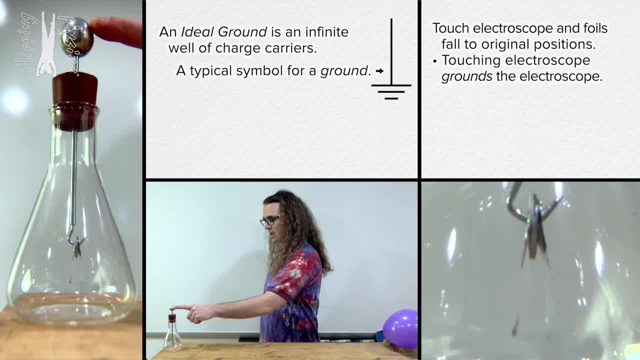 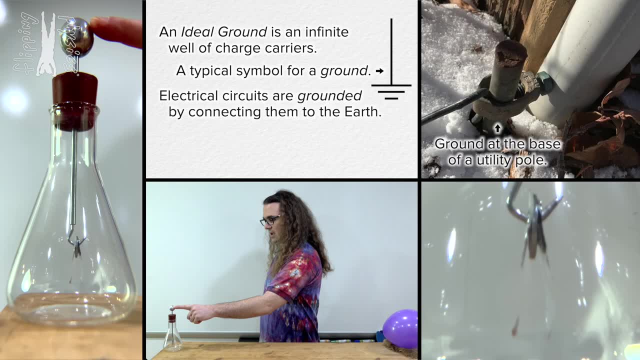 And this is typically the symbol used for a ground. I'm sorry what Mrp? Okay, sorry, I know it can be confusing. We call it a ground because electrical circuits are literally connected to the earth or the ground And the earth has, relatively speaking, an infinite number of electrons which we can. 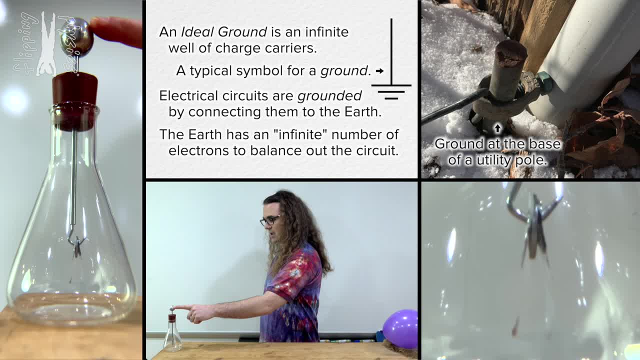 pull from it or we can give to it Again, relatively speaking. Relatively speaking, an infinite number of charges. If something goes wrong in a circuit, the ground will serve as a way to balance out the charges. In this example, when I touch the electroscope, the electroscope is no longer electrically. 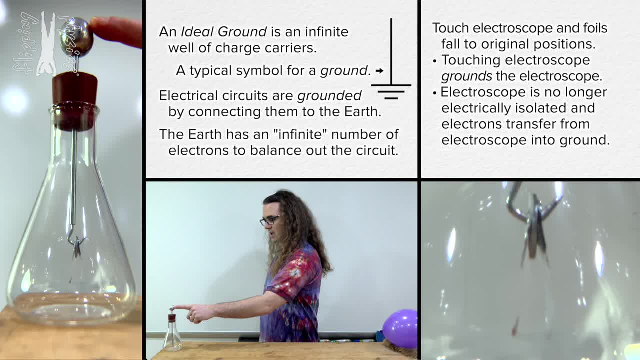 isolated and the excess electrons on the electroscope flow out of the electroscope into the ground, into me, And the electroscope is now electrically neutral, which is why the foils are no longer repelled from one another. Does that make sense? 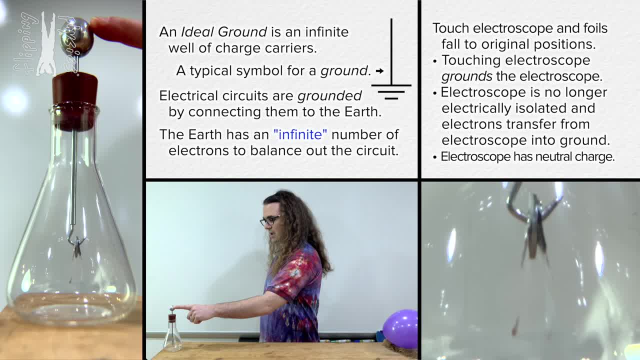 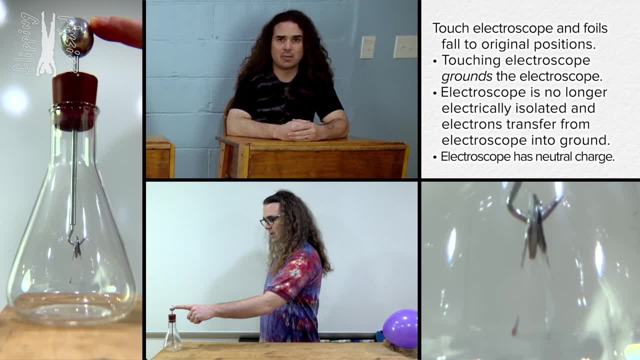 Yeah, I think it was the infinite term that confused me. What you mean is that you, as the ground, have so many more charge carriers in your body than the electroscope, such that you can take or give as many charges as necessary to cause the electroscope to become electrically neutral. 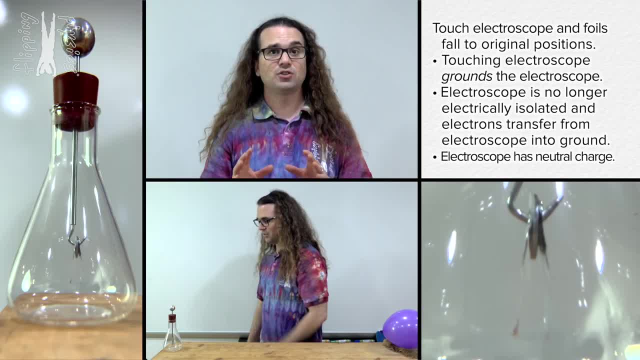 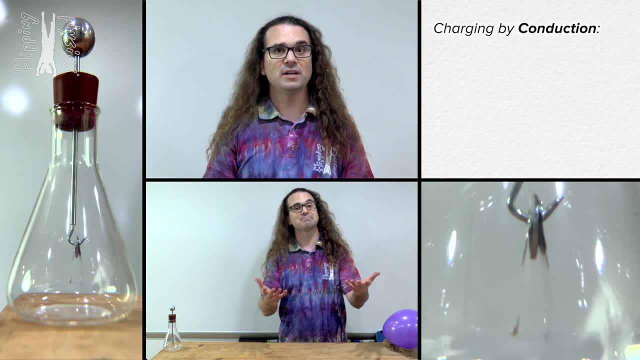 Right. Yes, Bo, That is correct. Okay, So that is charging by conduction. Two things I want to make sure you realize about charging via conduction. One is that the two objects have to be electrically neutral. Right. 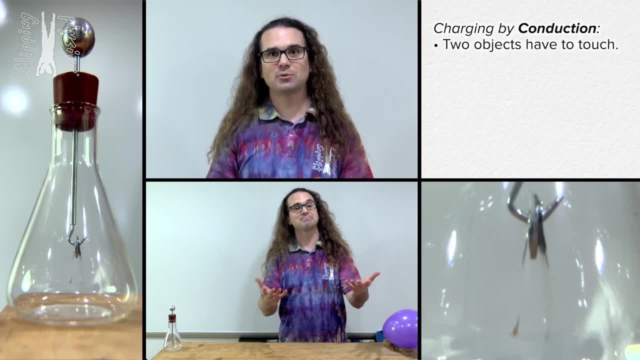 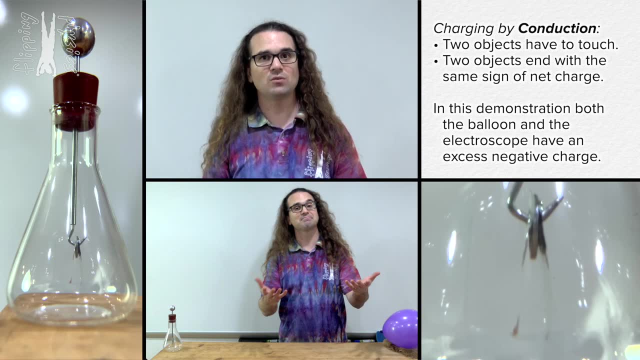 One is that the two objects have to touch, And two is that the two objects end with the same sign of net charge. In this demonstration, both the balloon and the electroscope end with a net negative charge, You mean before you ground the electroscope right. 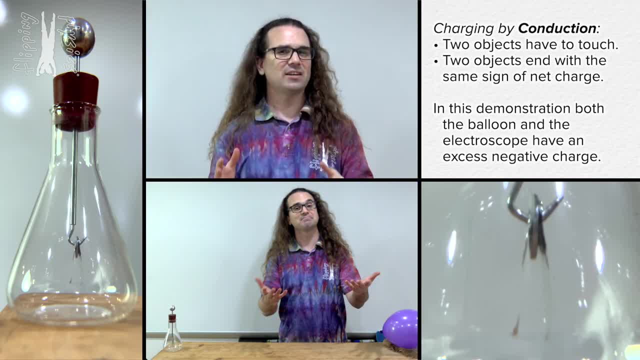 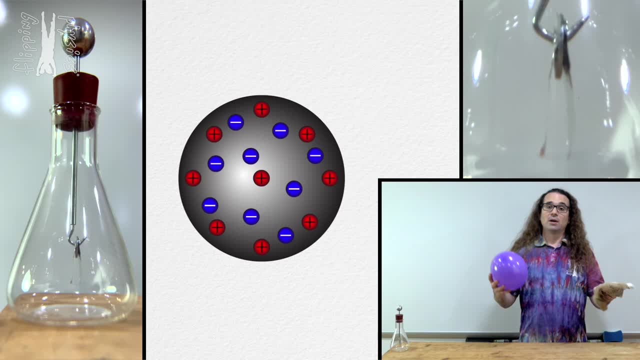 Correct, Bobby. That's before I ground the electroscope. Actually, let's watch the whole demonstration through once more. only this time I'm going to add typical idealized illustrations which go along with this demonstration. Rather than the electroscope, we have a neutral charge. 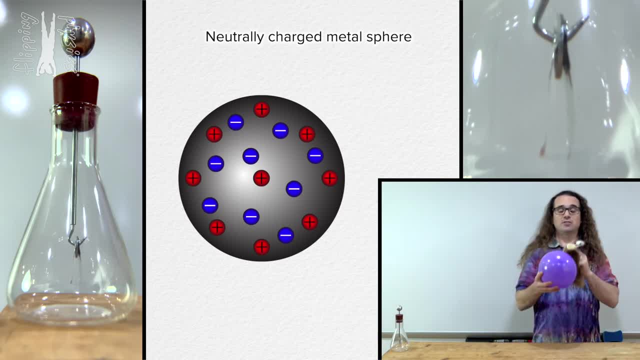 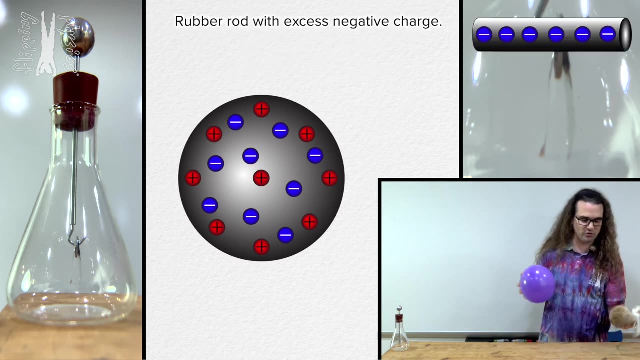 We have a neutrally charged metal sphere. Notice: the metal sphere has the same number of positively charged protons and negatively charged electrons. This is why the metal sphere, which represents our electroscope, is neutrally charged at the start. Then, rather than using a rubber balloon, we have a rubber rod with an excess of electrons. 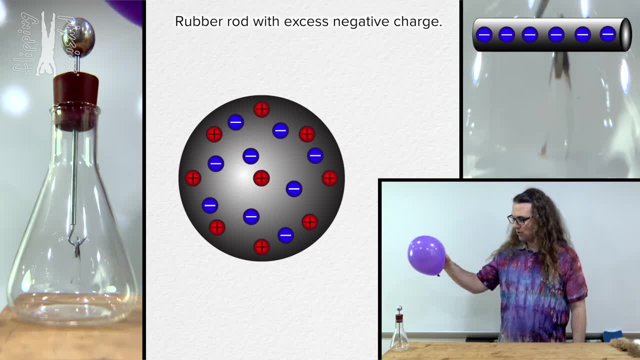 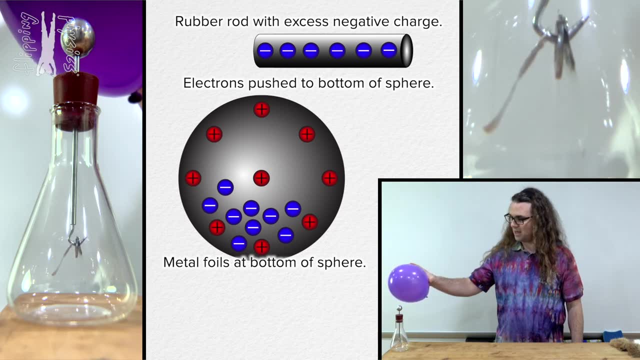 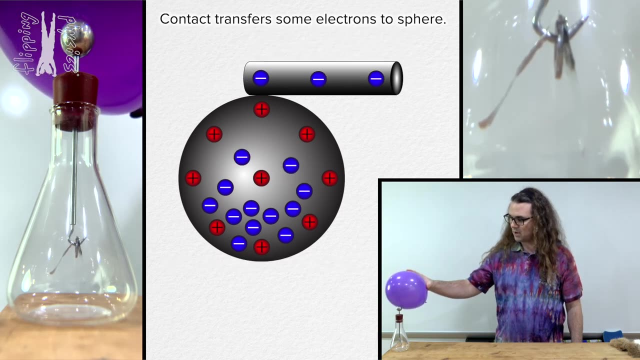 Bringing the negatively charged rubber rod near the top of the metal sphere pushes the electrons in the metal sphere closer to the bottom of the metal sphere or the bottom of the electroscope. This is why the metal foils are pushed apart. Touching the rubber rod to the metal sphere transfers some of the electrons from the rubber. 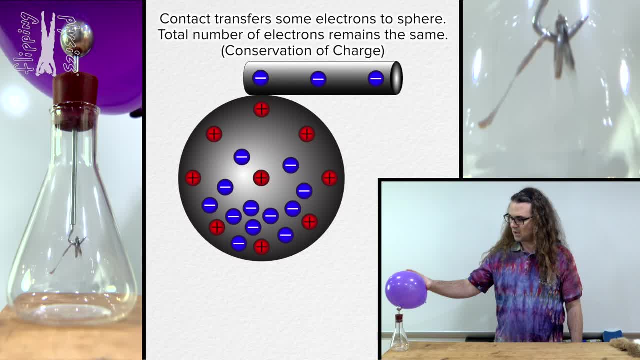 rod to the metal sphere. This decreases the number of electrons on the rubber rod and increases the number of electrons on the metal sphere. However, because of conservation of charge, the total number of electrons stays the same. Now we remove the rubber rod and the electrons in the metal sphere distribute themselves. throughout the metal sphere and the metal sphere has a net. And this is the summary. You might want to check out many other videos like this one. I'm going to go in a completely different direction next time. We are at the end of the video. 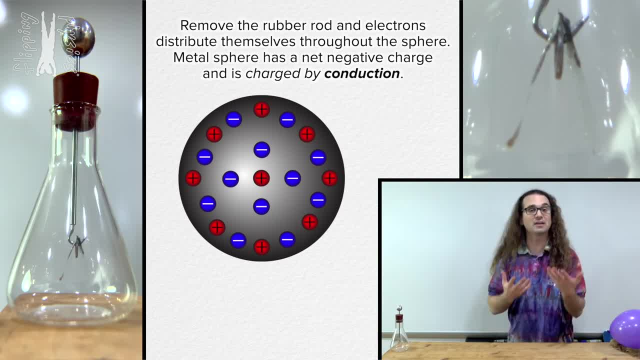 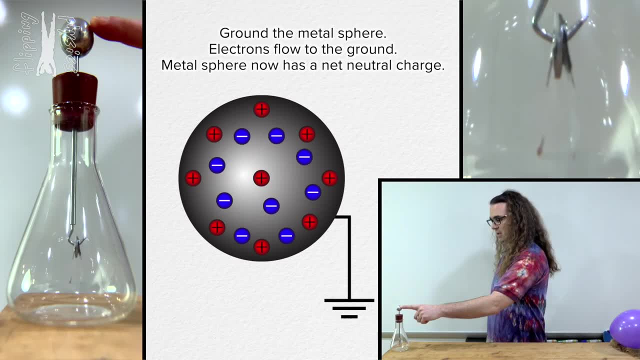 negative charge, which is why the metal foils are pushed apart from one another. now The metal sphere which represents the electroscope has now been charged by conduction. Then we ground the metal sphere, which allows the electrons to flow from the metal sphere. 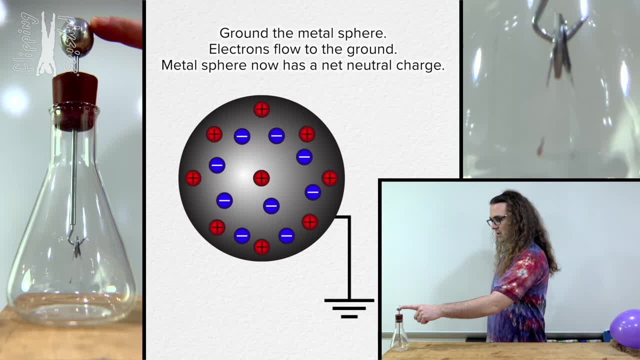 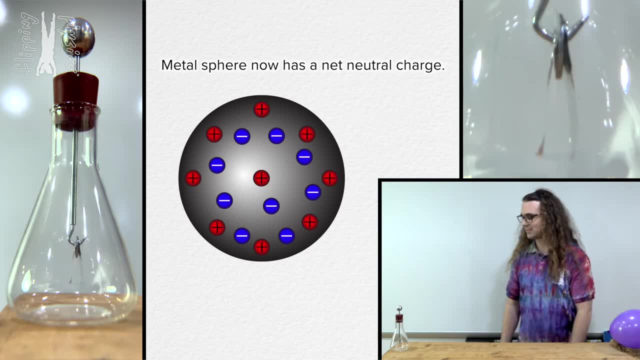 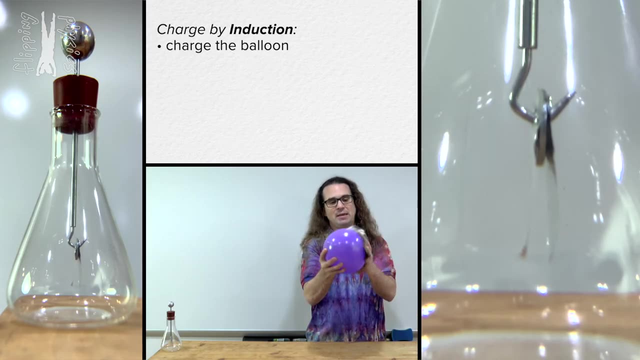 to the ground and leaves the metal sphere with a neutral charge. Okay, next let's demonstrate charging via induction Class. are we ready to demonstrate charging via induction? I am ready. Here we go Again. I charge the balloon by friction, by rubbing it against the rubber balloon. 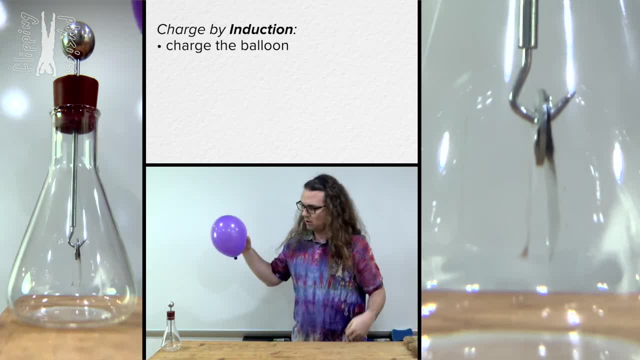 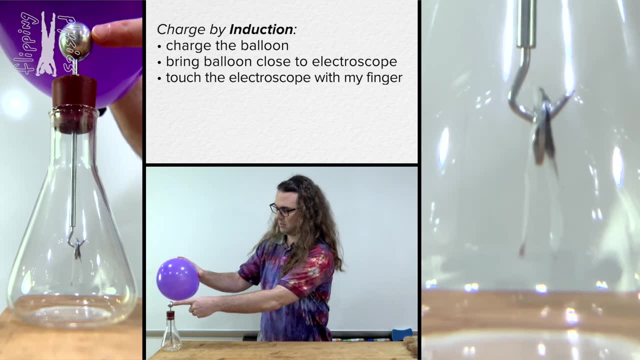 the fur, whatever. and then I bring the rubber balloon close to the electroscope, but I do not touch the electroscope. you can see the two foils move apart. Then I touch the electroscope, the two foils move down. I bring my finger away from the. 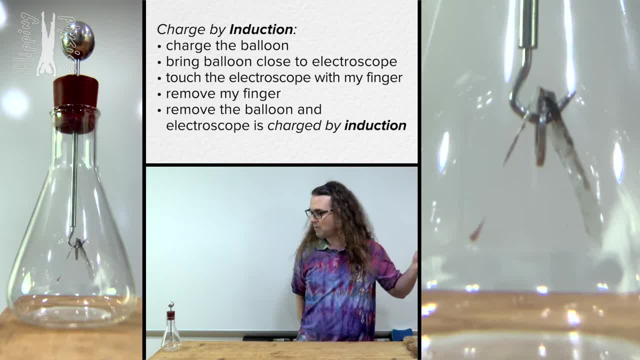 electroscope, and then I bring the rubber balloon away and the two foils move apart from one another and you can see the electroscope is charged via induction, And then I can again bring my finger in and ground the electroscope and the two foils move down next to one another. 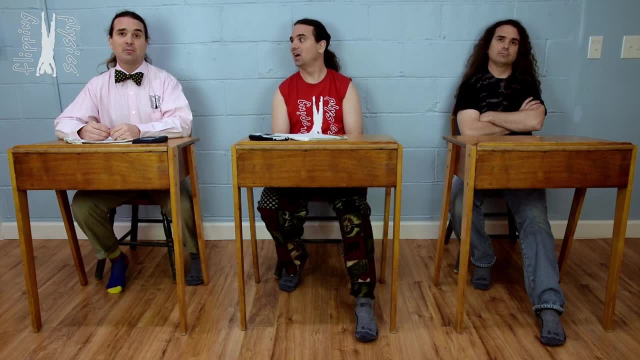 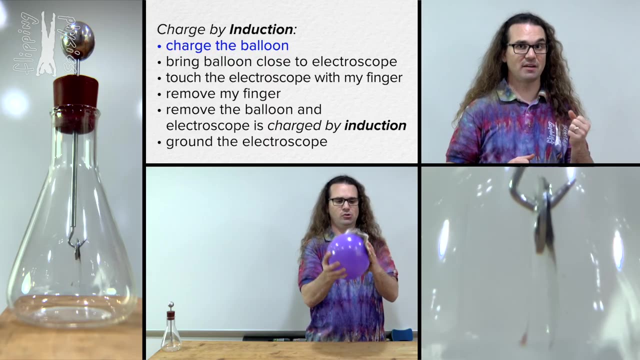 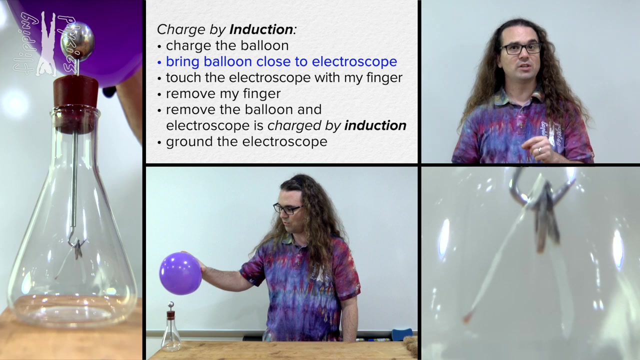 And that's it. Now we're going to walk through it step by step, right, because I really I need to. Yes, Step 1 was to give the balloon a net negative charge with an excess of electrons. Step 2 was to bring the balloon close to the electroscope but to not touch the electroscope. 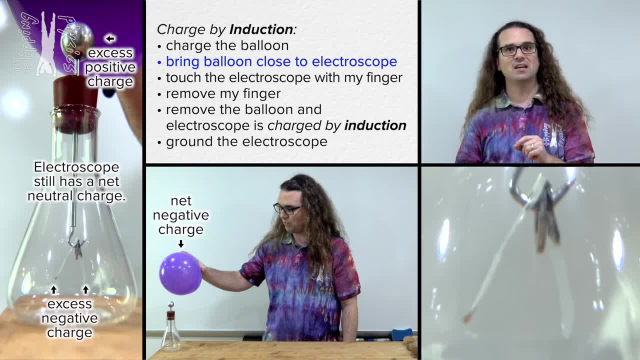 We determined in the last demonstration that the electroscope now has negatively charged electrons in the foils because according to the law of charges they are charged by electrons. They are repelled from the electrons in the balloon And we recall that the positively charged protons do not easily move because they are 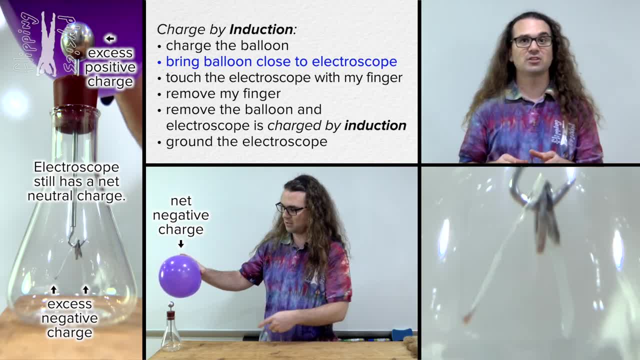 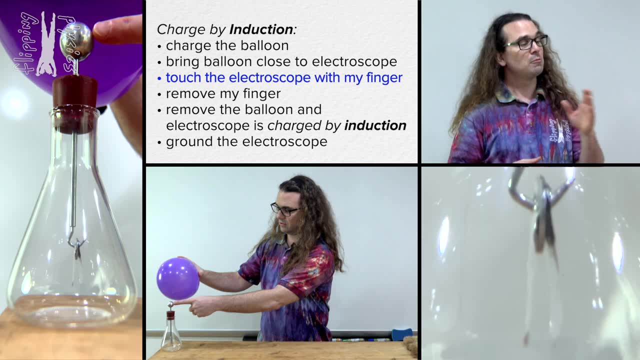 in the nucleus of the atoms. At this point the demonstration is different, because we do not touch the balloon to the electroscope. Instead, I touched the ball on the electroscope with my finger. Billy, what happens here? When you touch the electroscope, you act as the ground. 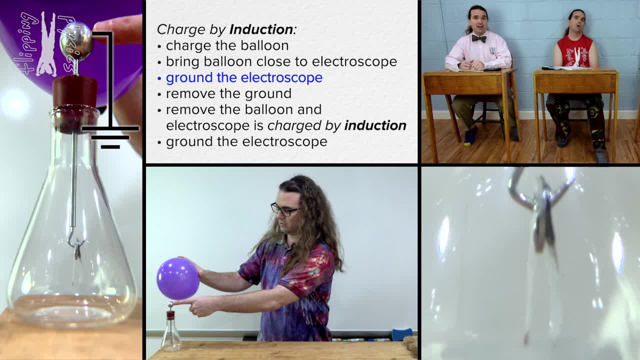 That means electrons in the electroscope are free to flow into the ground. They do that because, according to the law of charges, electrons are free to flow into the ground. They do that because, according to the law of charges, electrons are free to flow into. 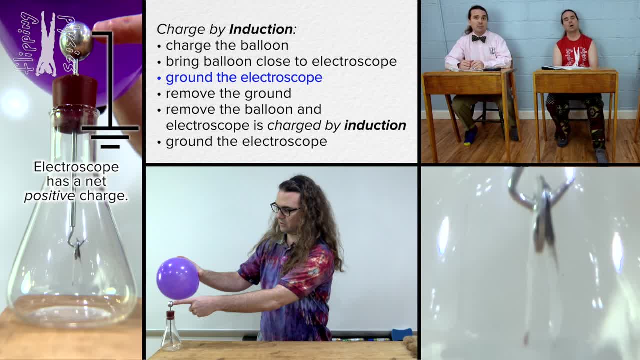 the ground. Light charges repel one another, so some of the electrons in the electroscope flow from the electroscope into the ground. They do this because you essentially provide an escape route for electrons to leave the electroscope. But there are still electrons in the electroscope- just fewer than before- and many are in the 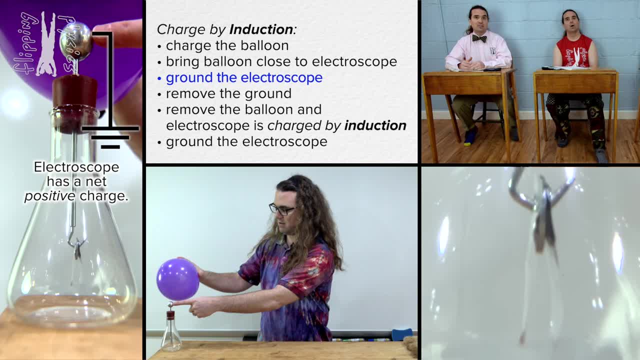 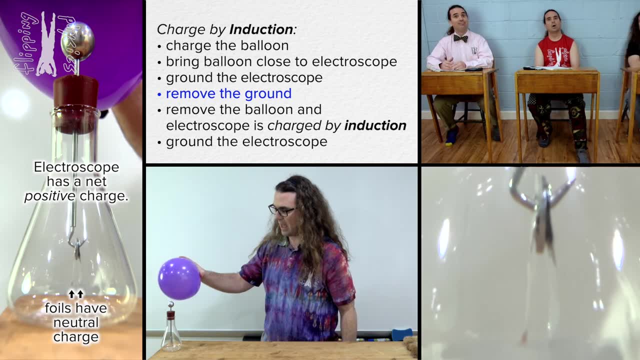 metal foils of the electroscope because they are repelled from the electrons in the balloon. That gives the metal foils a net neutral charge and the two foils are not repelled from one another. And then, When you remove the balloon, the electrons in the electroscope are repelled from one. 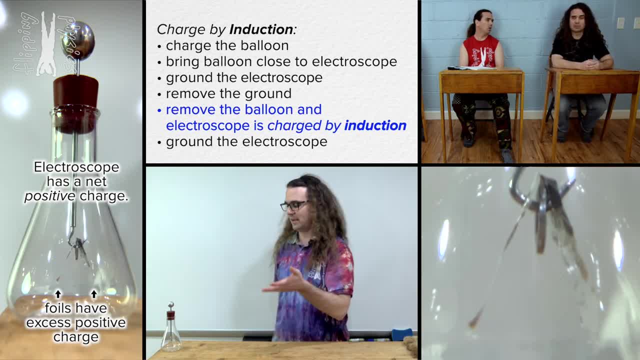 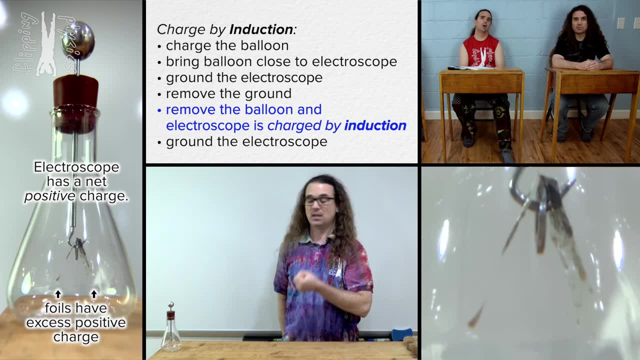 another in the electroscope and get distributed throughout the electroscope. That leaves the electroscope with an excess of protons and a net positive charge. That is why the metal foils are repelled from one another, because the positive charges in the foils repel one another. 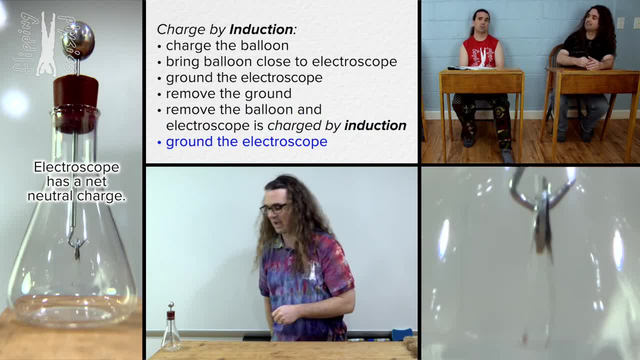 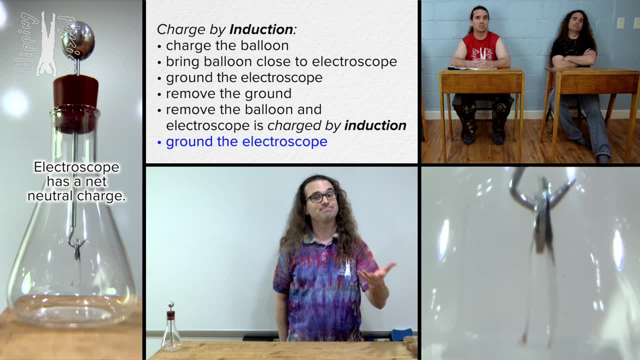 And then you touch the electroscope which grounds the electroscope. In this case that means electrons are pulled from your body into the electroscope to balance out the excess protons, And then you put protons in the electroscope and leave the electroscope with an equal number. 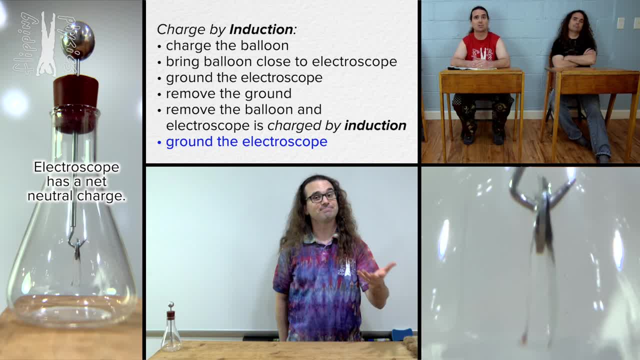 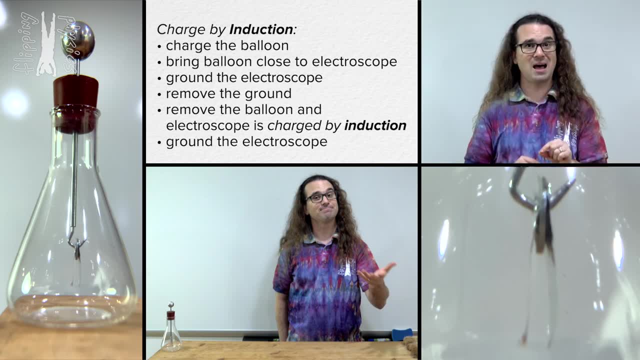 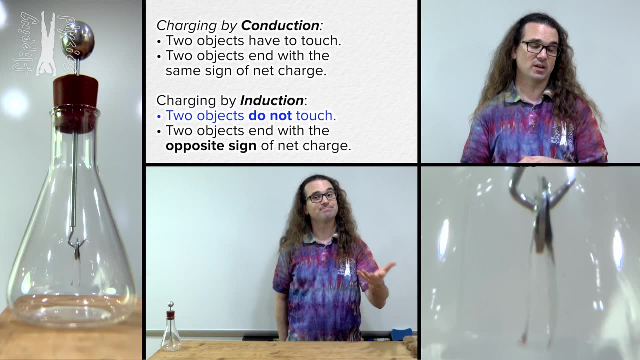 of protons and electrons and a net neutral charge. Exactly That is charging by induction. Again, there are two things I want to make sure you realize about charging by induction, and they are the reverse of charging by conduction. One is that the two objects never touch one another. 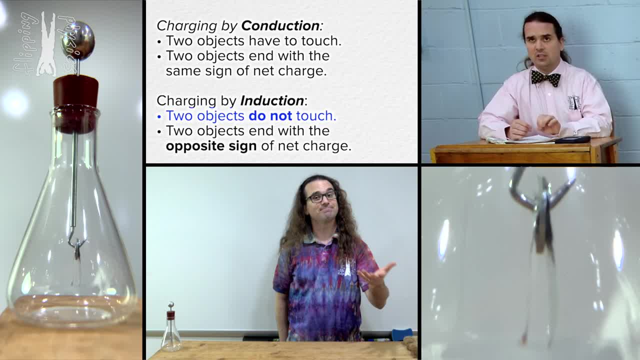 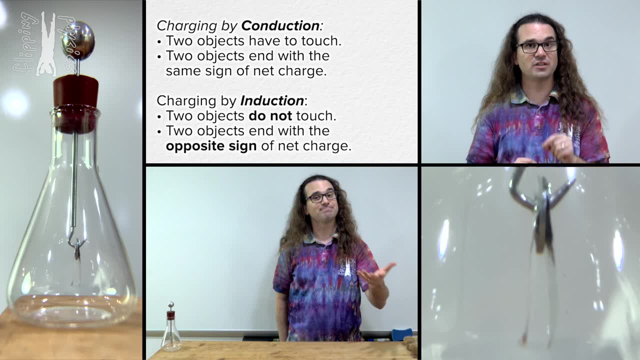 Okay, conduction: the two objects touch. induction: the two objects do not touch, they do not come into contact with one another. And two is that the two objects in this induction demonstration end with opposite net charges. In this demonstration the balloon ends with a net negative charge and the electroscope 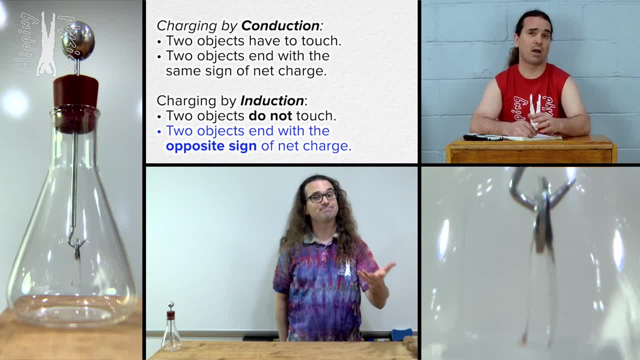 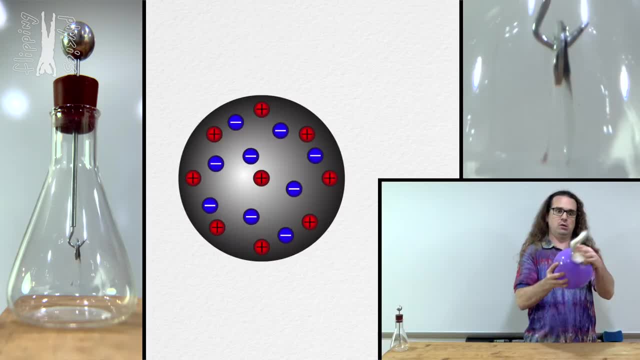 ends with a net positive charge. Again. this is before you ground the electroscope, right, That is correct, Bobby? again, before I ground the electroscope, Let's watch the whole demonstration through once more and again. I'm going to add the: